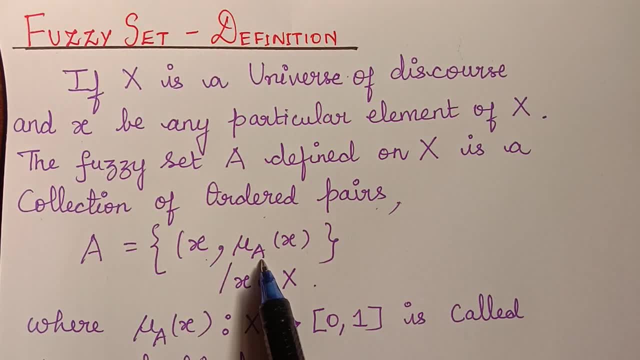 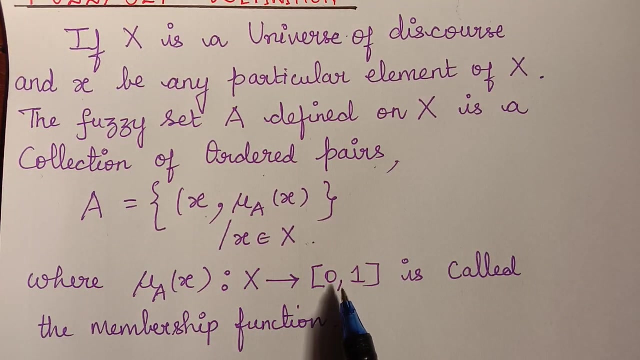 element of capital X and mu A of X is the membership value of X in the set A. So now A will be equal to the ordered pair X, mu A of X for all X belonging to capital X. So this is the definition of a fuzzy set and this membership value takes values in the interval 0, 1, that is. 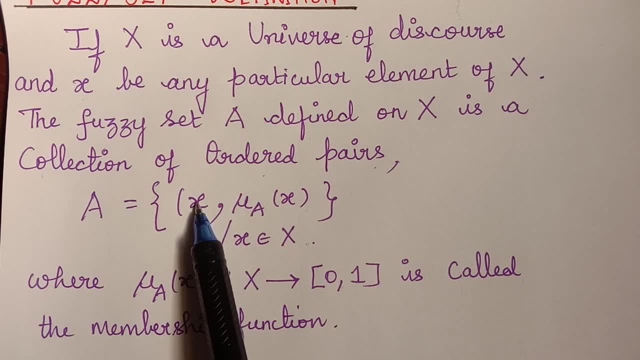 closed interval 0, 1.. It is a mapping of the elements to the closed interval 0, 1. that is, we consider all the points, all the infinite points between 0 and 1.. So we include 0 as well as 1 in that case where 0 represents no membership. 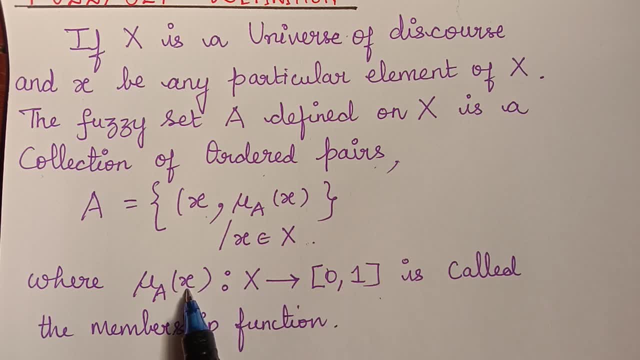 and 1 represents full membership. So this is known as the membership function, and we know that for a crisp set there is only two possibilities: either it can be 1 or it can be 0. So, but for a fuzzy set, the membership value is between 0 and 1.. In a crisp set, the function is: 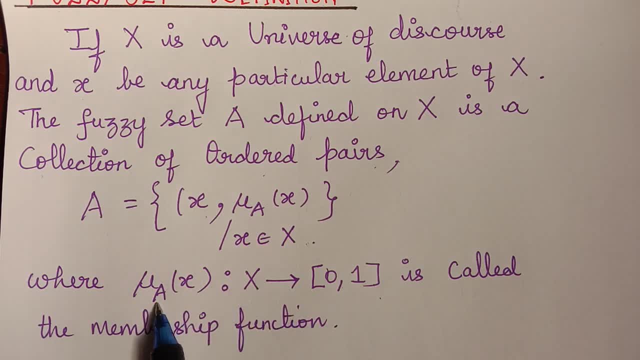 known as characteristic function, and here this function is known as membership function, as it represents the degree of membership of this element X with the set A. So this is the concept of fuzzy set. Now let us learn this with the help of an example. Now we consider a universal set. 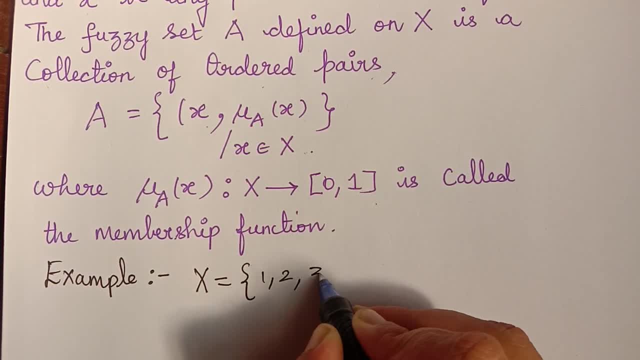 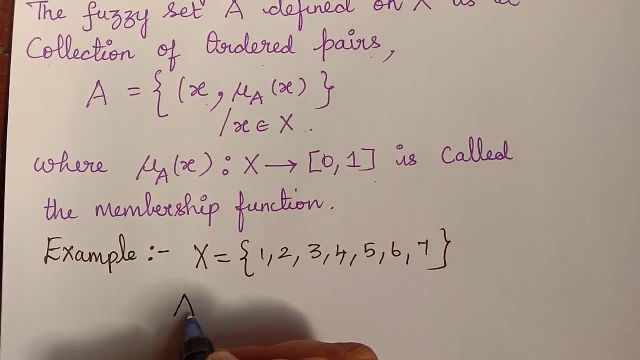 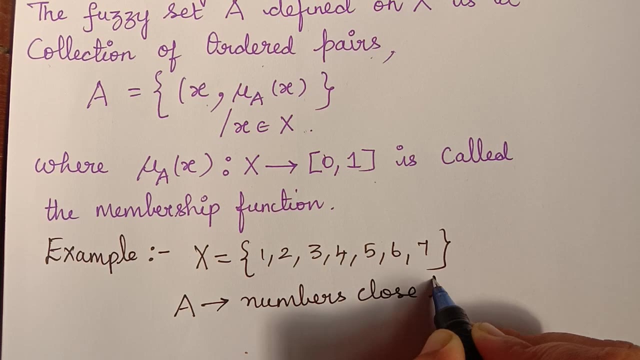 X equal to 1,, 2,, 3,, 4,, 5,, 6 and 7, and we consider the fuzzy set to be A and we consider the set to be numbers close to 3.. So in this universal set, we are considering the fuzzy set A, which 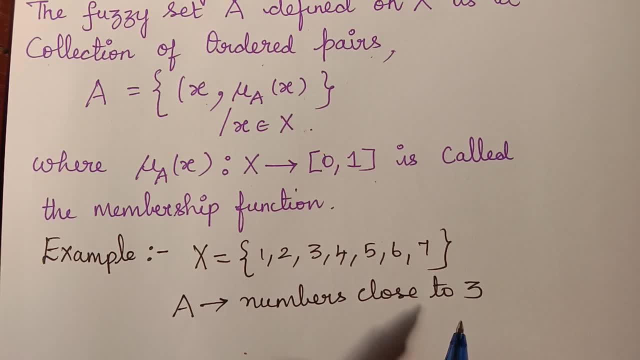 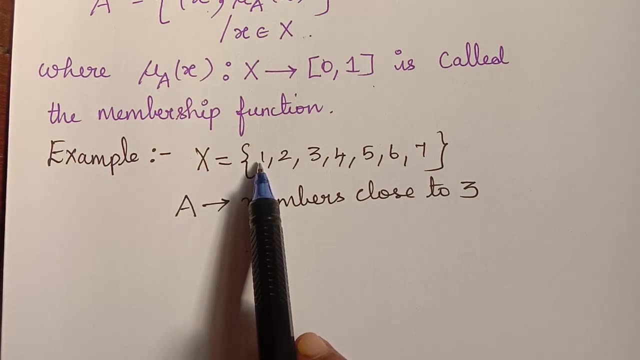 is considered as numbers close to 3.. We follow the notations as per the prescribed textbook And the notation for the fuzzy set. we are using it as A. Now we have to evaluate this set. Now we shall see that we notice that the universal set has numbers from 1 to 7.. Now, for each number, we 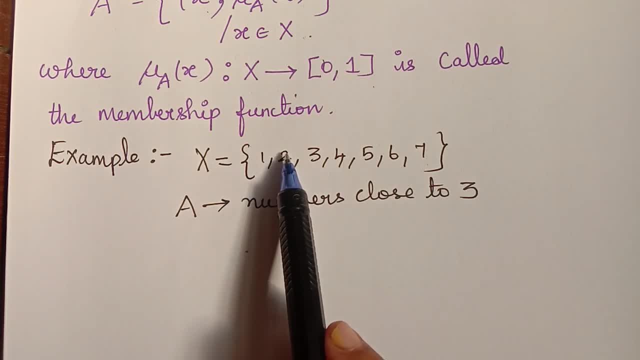 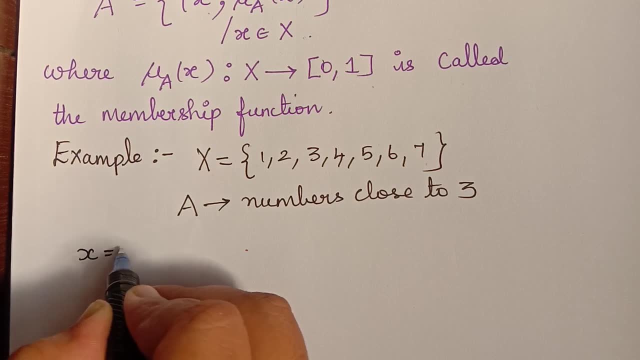 have to find the membership value as per the degree of its closeness to the number 3, and we have to write it here. For example, if X is equal to 1. So we can say that 1 is somewhat closer to 3.. 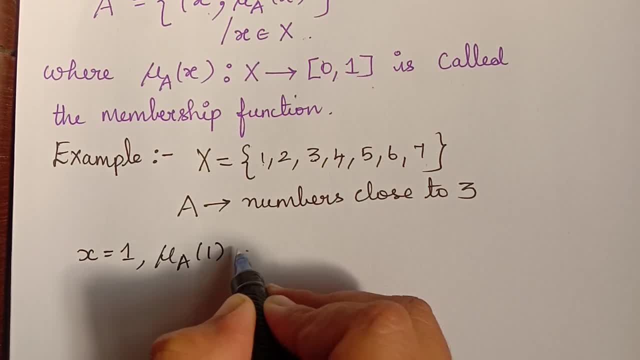 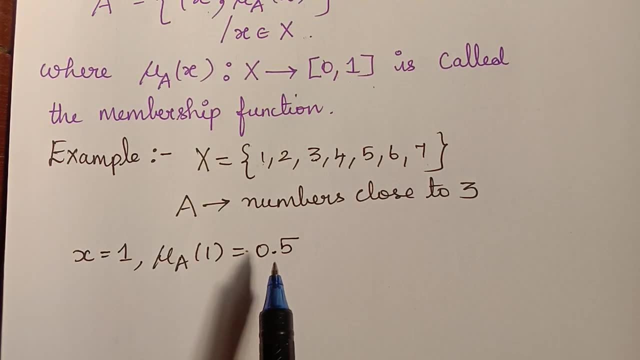 So we can have the membership value for 1 is to be equal to some 0.5, and this is absolutely manual. It may differ as per the view of the person, but it may not differ too much, also because this number is quite close to 3.. And now we have X to be equal to 2 and we find that this 2 is 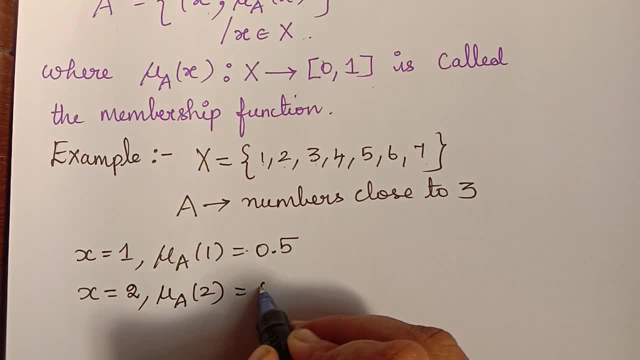 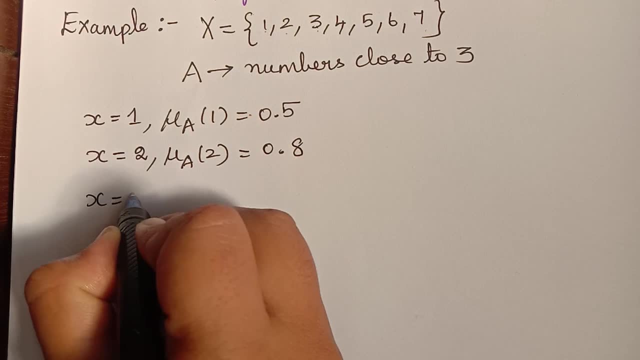 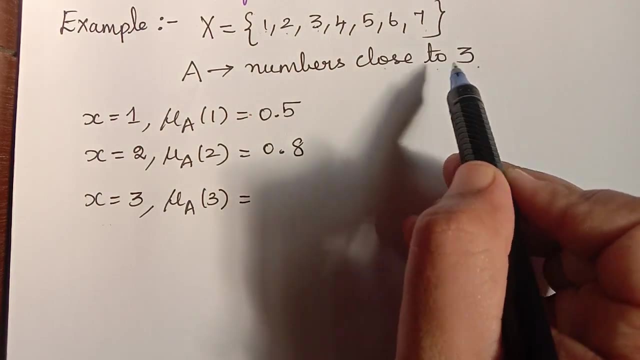 more closer to 3.. So we can have the membership value to be some 0.8.. And now next, let us evaluate. the membership value for X is equal to 3.. We find that we know that 3- the numbers close to 3 they are asking, but we have considered 3 itself. So definitely the membership value is. 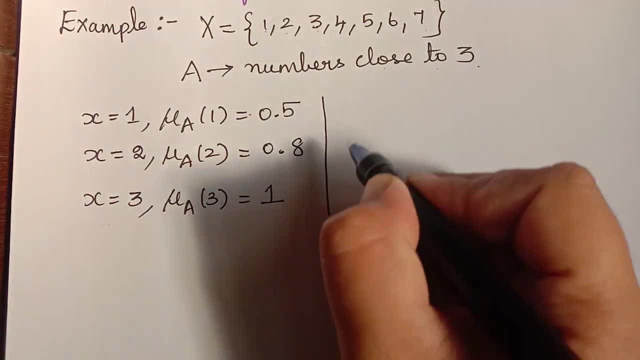 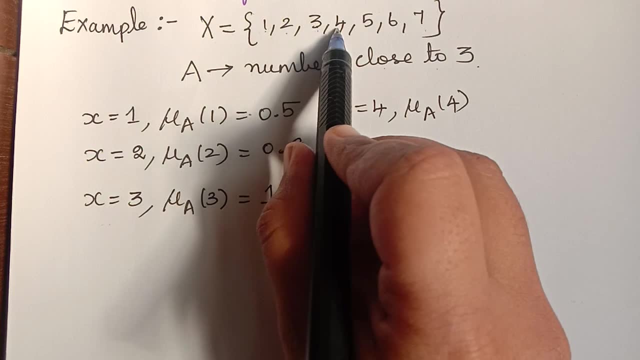 full, So it is equal to 1.. So for now, for example, X is equals to 4. we have to consider So the membership value for 4, how closer it is to 3. it is same as how closer 2 is to 3.. For 2 we have 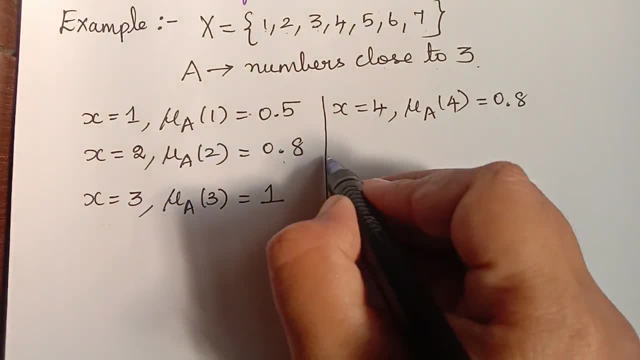 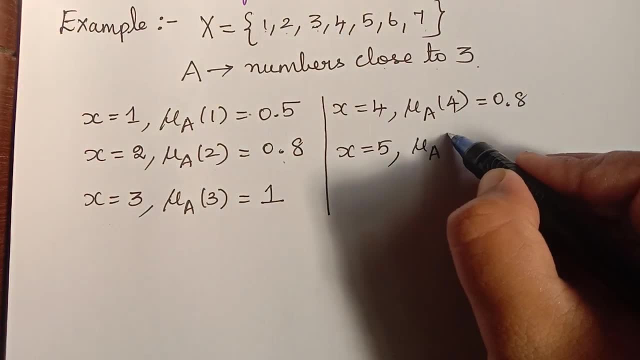 taken it to be 0.8, and for 4 we have taken it to be 0.8.. So we have taken it to be 0.8 and for 4 also, we will take it as 0.8.. And for X is equal to 5. it is same as how closer 1 is to 3.. So the 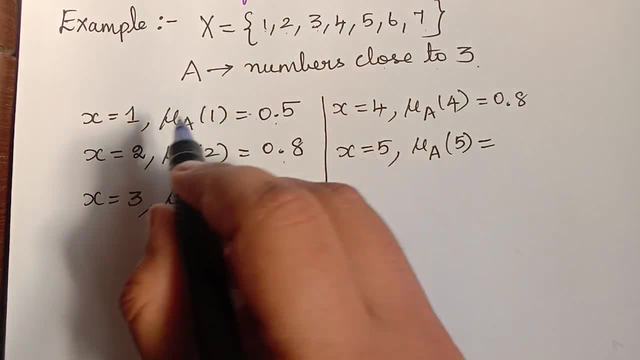 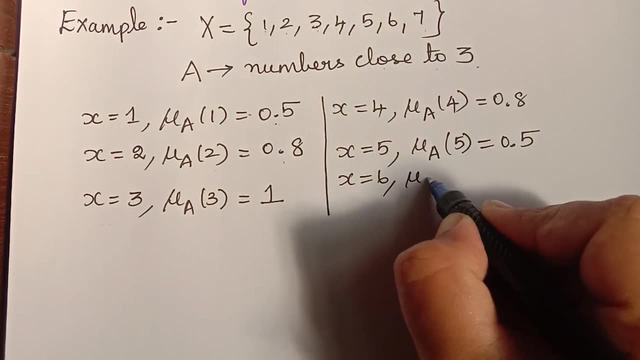 membership grade for 5 will. we can have the same one as we had for 1, and so we can have it as some 0.5.. Now let us take X. is X to be equal to 6. So it is more far from 3.. So the membership grade of. 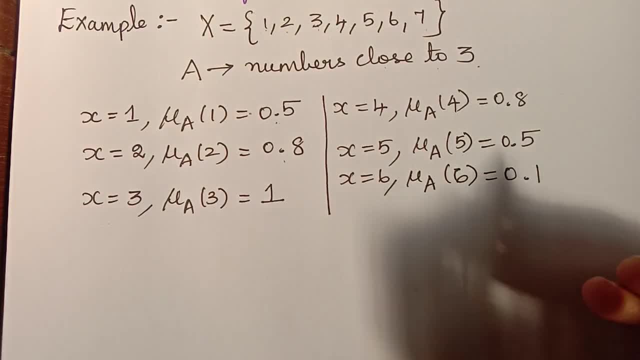 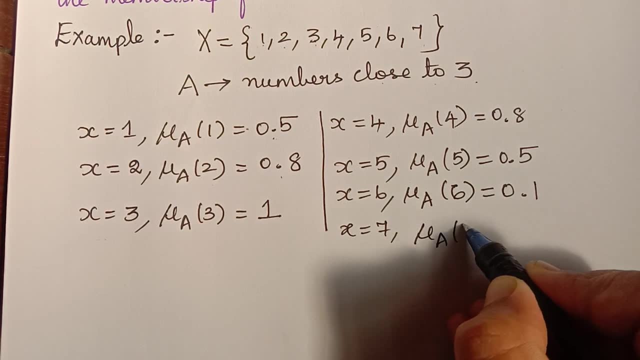 6 will be equal to. maybe we can have some 0.1.. Now next we have to take X to be equal to 3.. So the membership grade of 7 becomes more far from 3.. So we can take the membership grade to be.